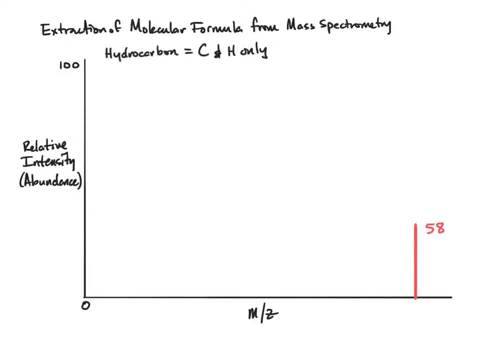 So, therefore, the first thing we want to do is determine the maximum number of carbons present in 58.. So what we can do is take the number of carbons present in 58 and put them in the molecular formula. take 58 and divide by the atomic mass of carbon, which is 12, so the max number of 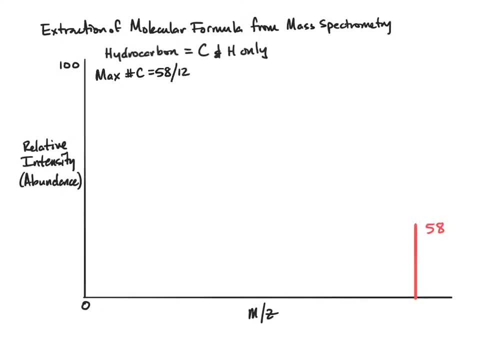 carbons is equal to 58 divided by 12 and you get 4.83. so we have to have a whole integer number. and is a meaning of logic in solving this type of problem. you're not going to round up to the next highest integer and there's a reason for. 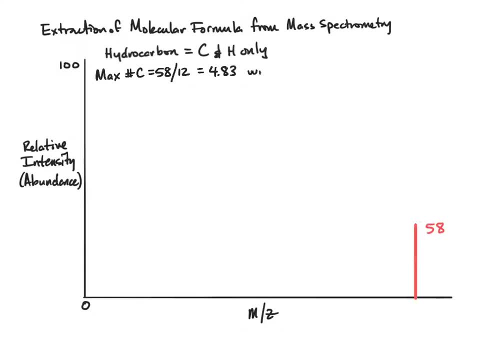 that. so the maximum number will be 4. the reason that it cannot be 5? because if we take 12 times 5, we end up with 60, and 60 is greater than 58 and we've already overshot what the data that we're given. so, again, because this is a hydrocarbon. 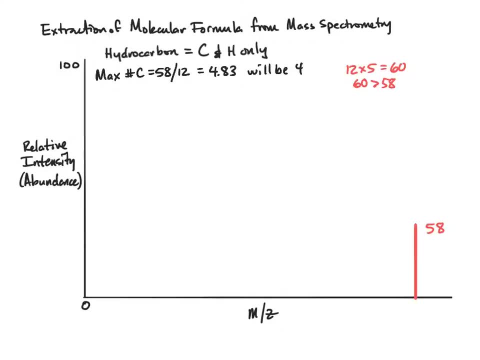 with carbon and hydrogen. it not only has to have carbon, it also has to have hydrogen. so if we're greater than the data point, we're given that that cannot be the maximum. so we're going to stick with 4 as the maximum number of carbons. so now what we want to. 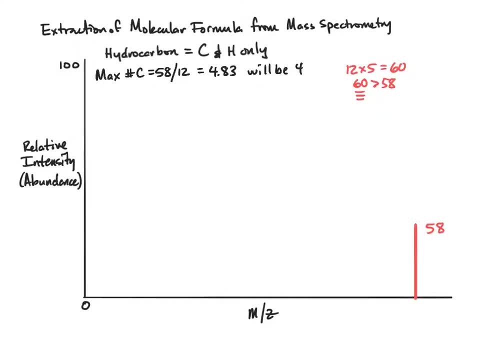 do is determine the carbon contribution. So if we take 12 times 4, that equals 48.. 48- those mass units belong to carbon. so therefore, what is the hydrogen contribution? it's going to be simply the difference. 58 minus 48 equals 10. 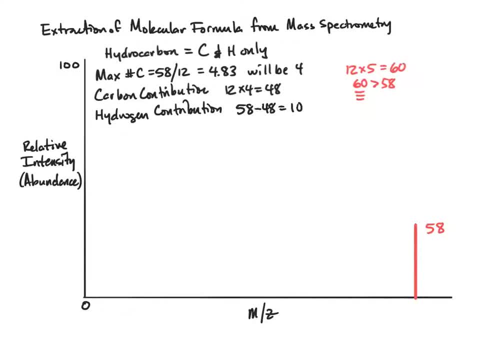 So we can see that, using this logic, we have 4 carbons and we have 10 hydrogens. So therefore, our molecular formula is C4H10.. Now to propose constitutional isomers, the first thing we have to do is determine if that molecular formula 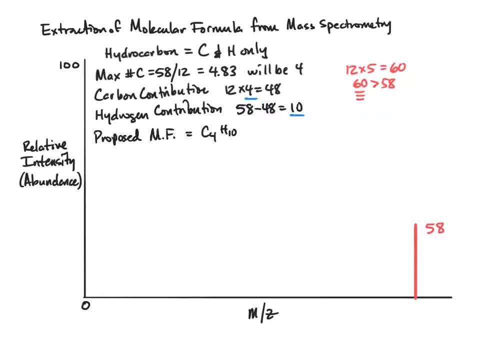 has any degrees of unsaturation. So remember, we're going to use CnH2n plus 2. That belongs to a saturated alkane. In our case, n is equal to 4.. Okay, Okay, So we end up with C4H10.. 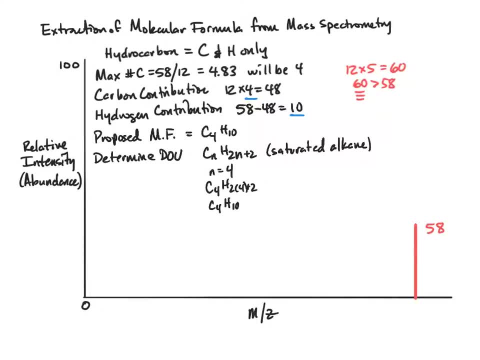 So for 4 carbons- that's what it should- be fully saturated, And we see that from our proposed molecular formula, C4H10,. we subtract these And essentially we end up with 0 degrees of unsaturation. What does that mean? 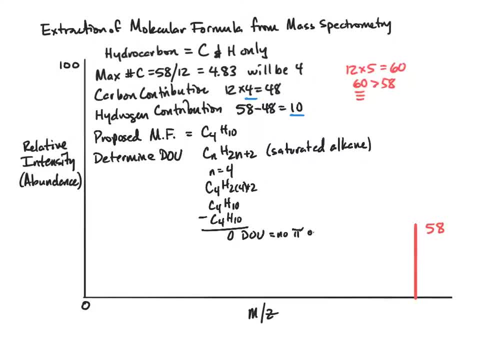 There are no pi bonds or rings present in the molecule, So every carbon is fully saturated. That means all carbons are sp3 hybridized, So we can go ahead and start proposing structures for this constitutional isomers. We have 4 carbons. 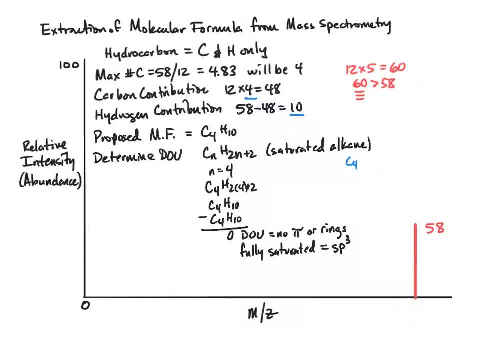 So the first one is C4H10.. And the first thing we can do is put them in a row. So there's 4 carbons. That's linear. That's going to have 2 unique carbons, 2 unique type of hydrogens.